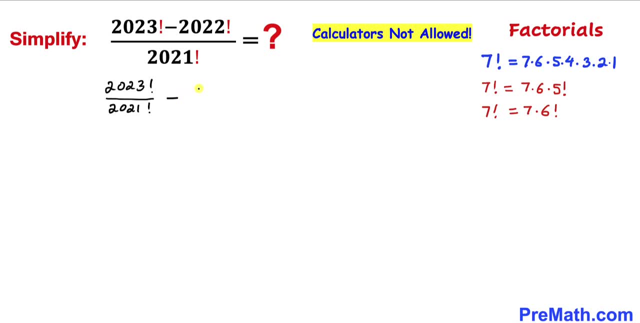 factorial, and then minus 20, 22 factorial, divided by 20- 21 factorial. let's go ahead and simplify this one and the numerator 22, 23 factorial, and this could be written as 20, 23 times 20, 22 and then times 20. 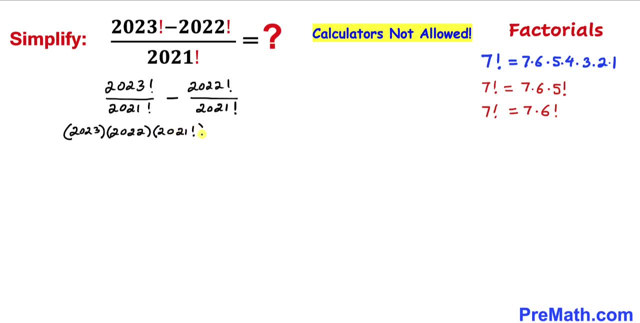 21 factorial, divided by this 20- 21 factorial and minus. and now let's focus on this numerator, 22, 23 factorial, and this could be written as 20, 22 times 20- 21 factorial, all over 20, 21 factorial. and now we can see this: 20- 21 factorial cancels out. 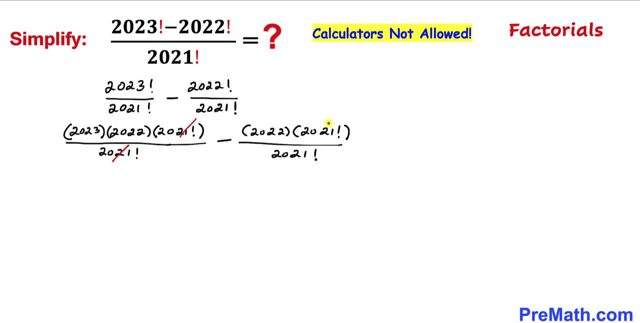 with this 20 21 factorial, and likewise, this 20 21 factorial cancels out with this 20 21 factorial as well. so therefore, we are ended up with the 20 23 times 20 22 minus. here. we are just left with this. 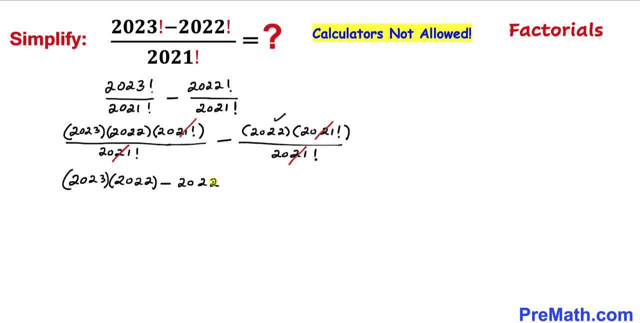 20 22, and here we can see 20 22 and 20 22. they are in common, so therefore we can write 20 22 outside and we got 20 23 minus 1, and now we can see 20 22 could be written as 2 times. 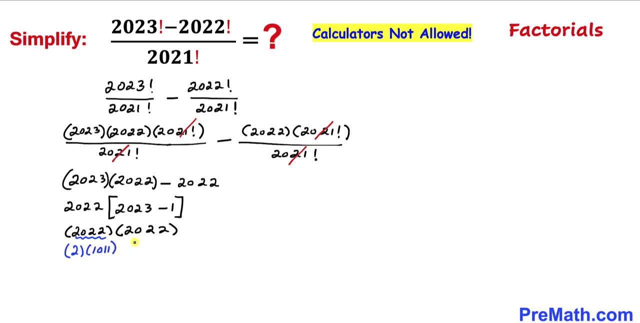 10, 11, 1011. likewise, this could be written as 2 times 1011 as well, as you can see in this next step. now let's go ahead and multiply 2 times 2 is going to give us 4, and let's multiply these one as well.